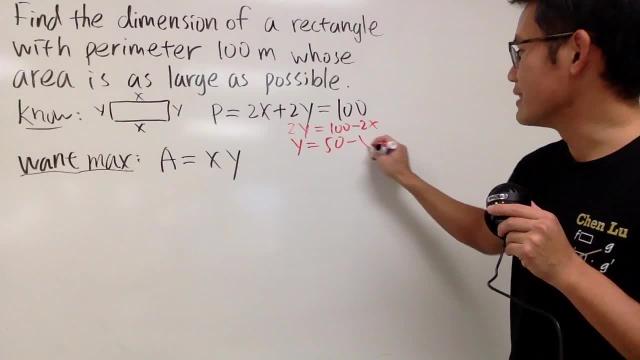 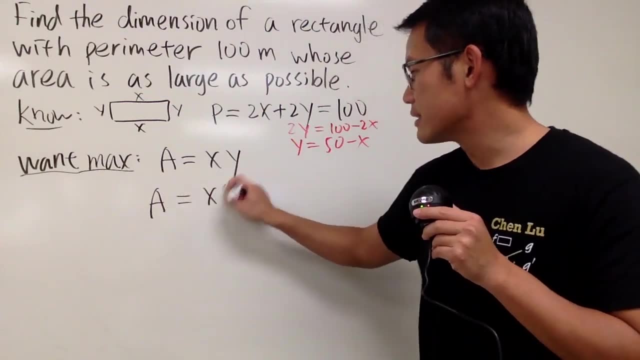 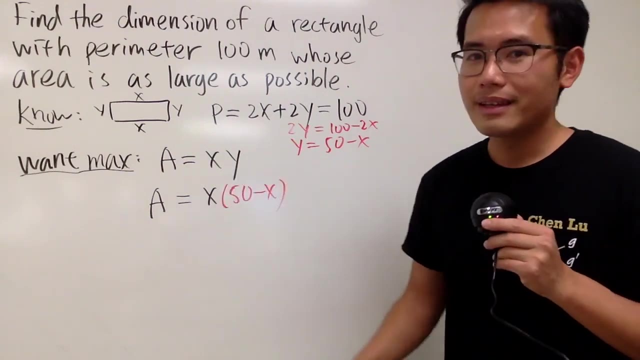 everybody by 2. So y is equal to 50. Minus x. Very nice, huh? Then put this right there. So we see a equals x times and the y is just 50 minus x. Very nice, And this now is just a function of x. I will just call this to be x. 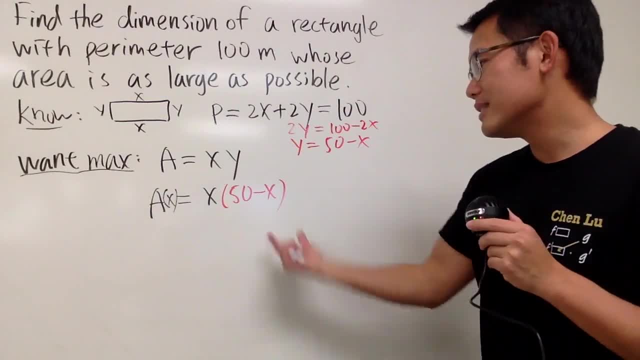 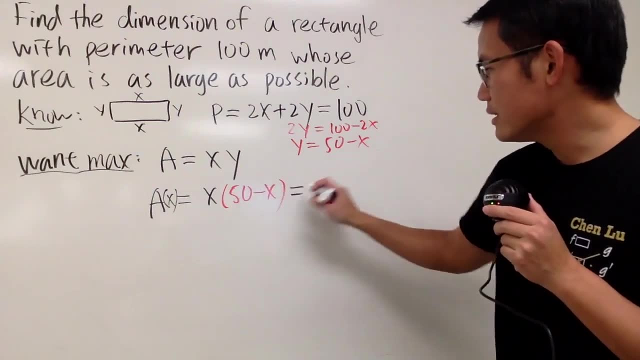 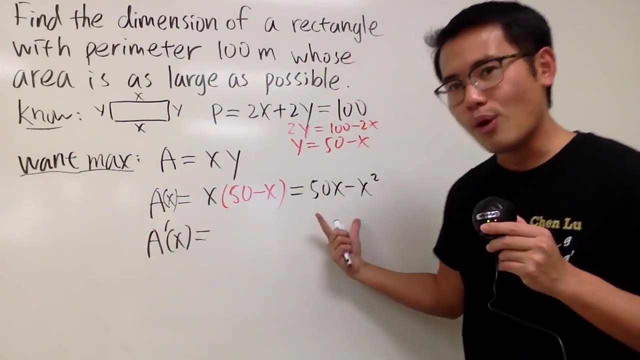 a of x, a of x, And this is quadratic. but we'll do calculus even though we have a nice formula for that. Anyway, you see that we can actually multiply this out. This is 50, x minus x squared, And let's go ahead and do our derivative. But look at this form: 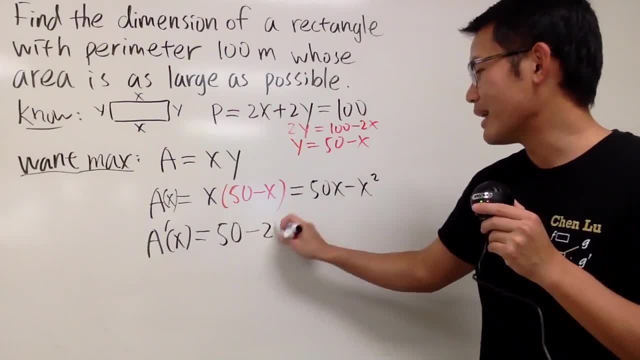 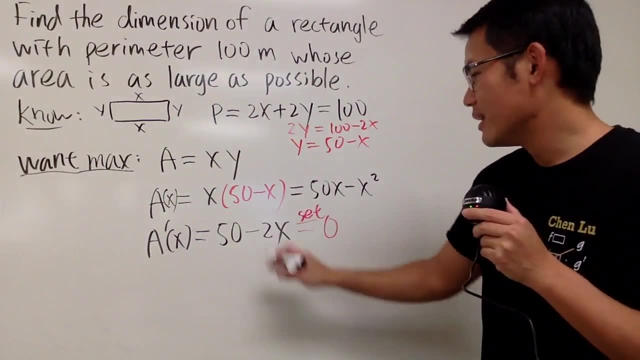 Differentiating this, we get 50.. Differentiating that, we get minus 2x, And, of course, set this to be 0. And solve this right. Do whatever you need to do, you will get x is equal to 25. And that's. 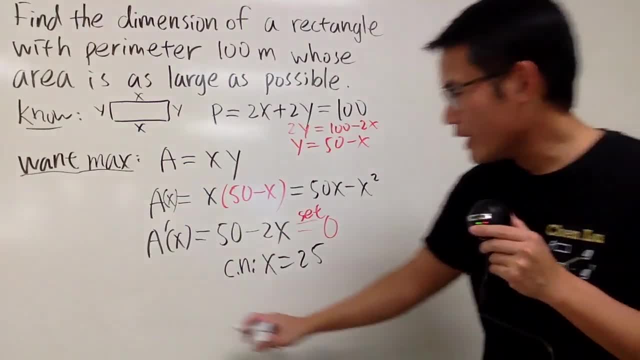 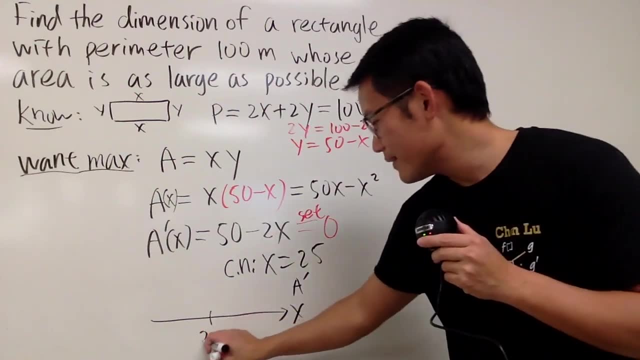 going to give you the critical number, And that's very nice. Have a look, When we have the x value prime 25 right here, Pick a number less than 25.. Let's say 10. Put it here: You get a positive. 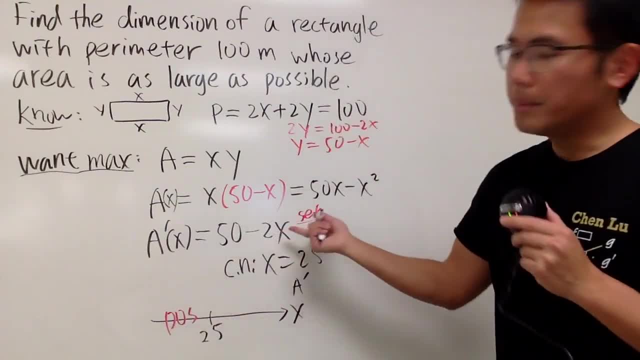 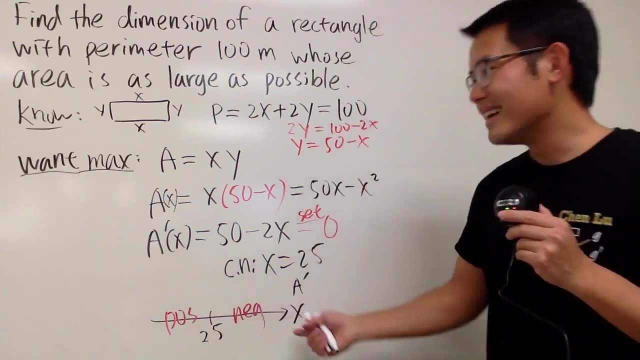 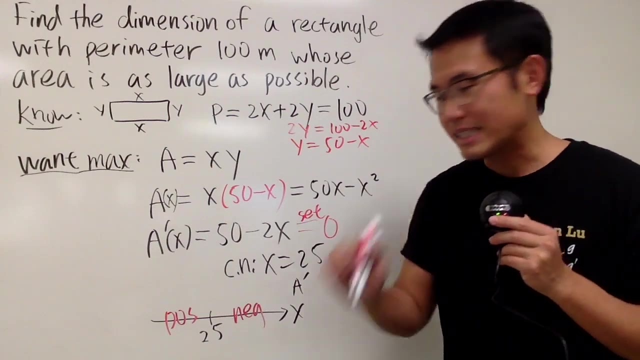 right. So this right here is positive: Pick a number bigger than 25. You get, let's say, 27.. You get negative. So this right here tells us our function is going to be increasing and then decreasing. So that means, right here, we have the maximum right. So I will just indicate that this. 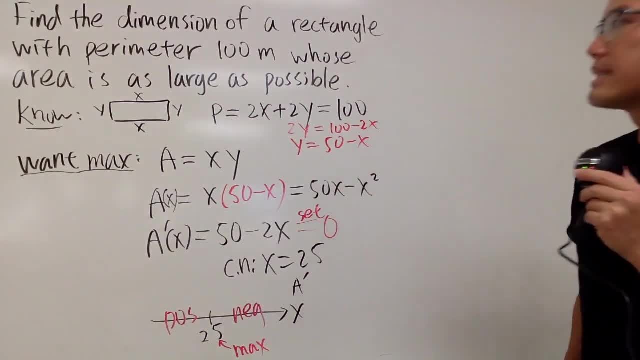 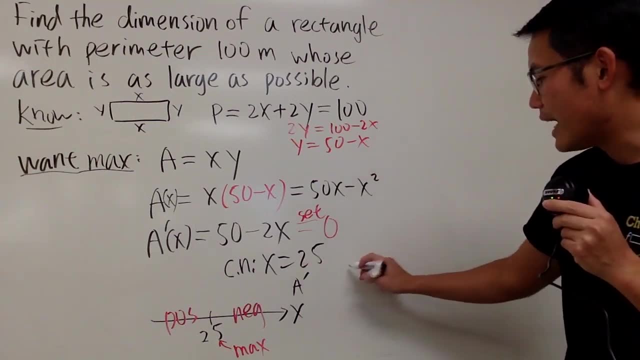 right here. It's indeed a maximum. Now the question is asking us to find the dimension, So we just have to find out what y should be as well. We know x is 25.. And that means y is equal to 50 minus x, And of. 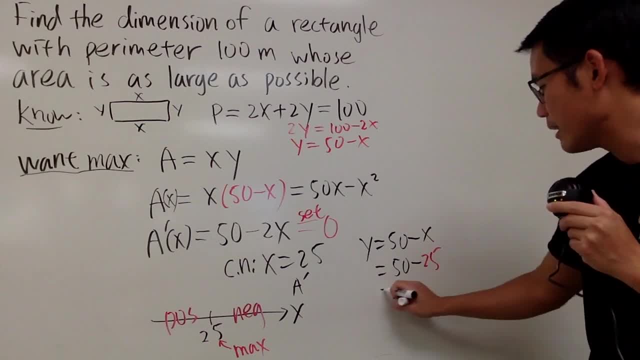 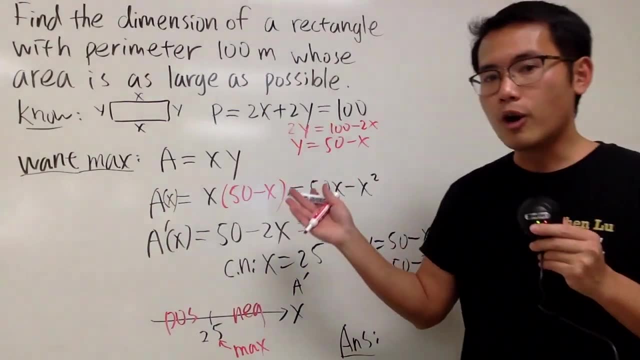 course that's just going to be 50 minus 25.. And that means y is equal to 25.. Just like that. So this is how we can answer the question. We want the rectangle to be 25 by 25.. So just say 25. 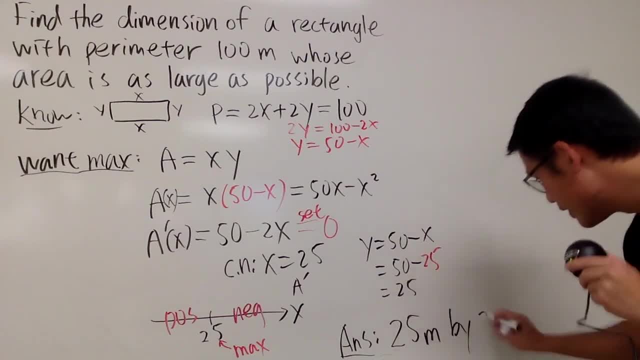 meters. We're talking about length right here By 25 meters. So this right here is it.